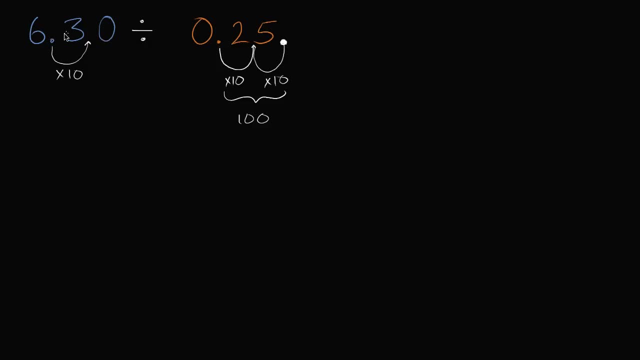 Or we could actually add as many zeros as we want to the end of this and not change the value. It's still 6.3.. 6 and 3 tenths is the same thing as 6 and 30 hundredths, So now I can move the decimal one more spot to the right. 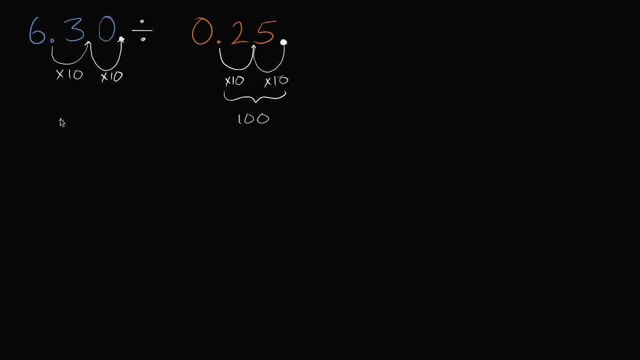 And so I'm multiplying by 10 again, And it becomes 630.. So 6.3 divided by 0.25 is the same thing as 630 divided by 25.. Let me do that again, because this is really the tricky part. 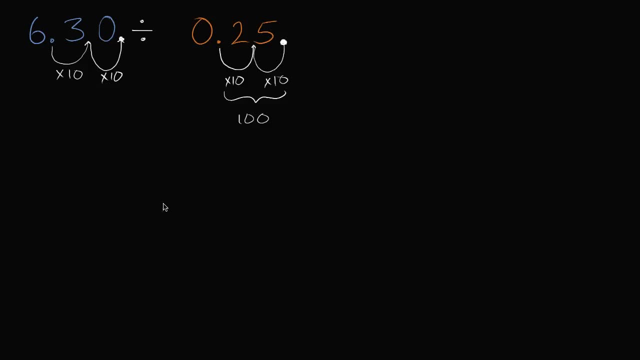 or the artful part when you're dividing decimals. If I were to write 0.25 being divided into being divided into 6.3. Six, let me do it: Six, 6.3. Now, what I care about is moving this decimal. 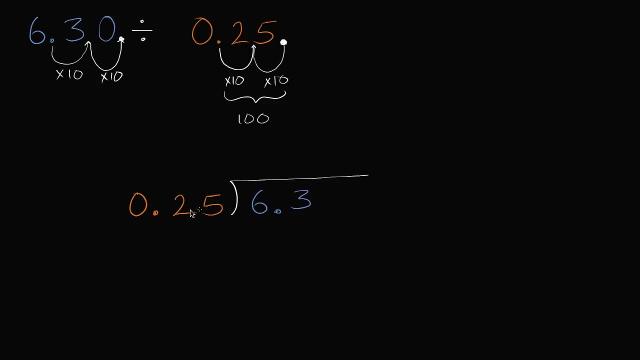 to the right. far enough so that this becomes a whole number. I don't have to move it any further, just far enough, so this becomes a whole number. And then I have to move this the same number of times to the right, But the goal is to make this a whole number. 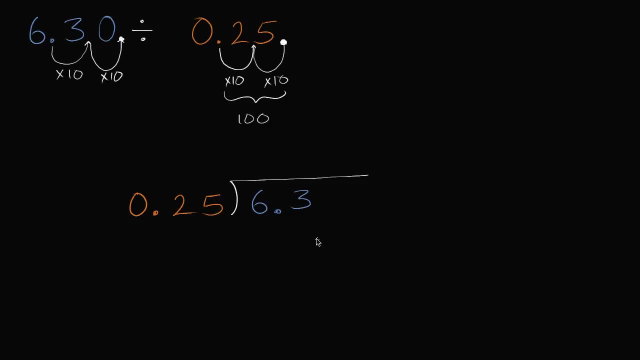 not to make the 6.3 a whole number, although that is going to happen for this particular case. So if I move it two spaces to the right, so one, two, 0.25 becomes 25.. And then 6.3 becomes. 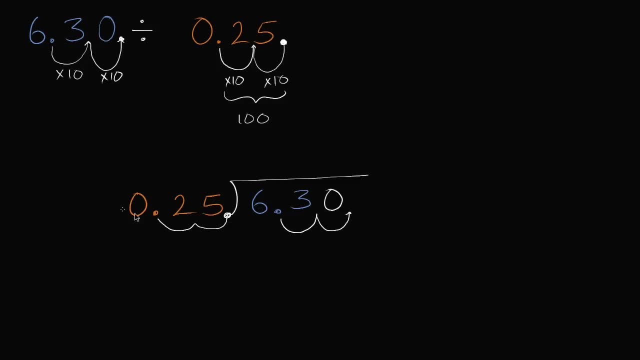 move it one space, two spaces to the right, it becomes 630.. And so let me clarify that, Let me just clear all of this stuff out of the way, to just make that clear what I just did, so we don't have to deal with all this messiness. 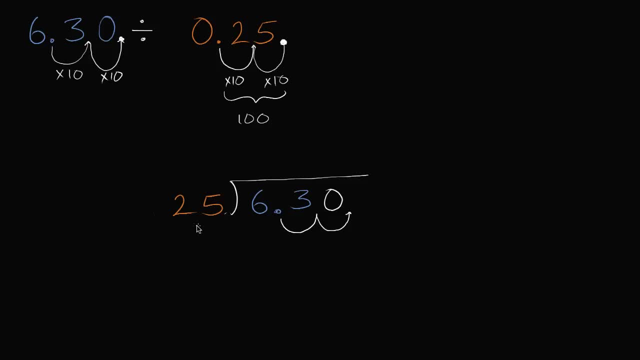 when we're actually doing our long division now, And so this one over here. let me erase all of this business. And we are ready to do some. we're ready to do some long division, All right, So now, this is just straightforward. 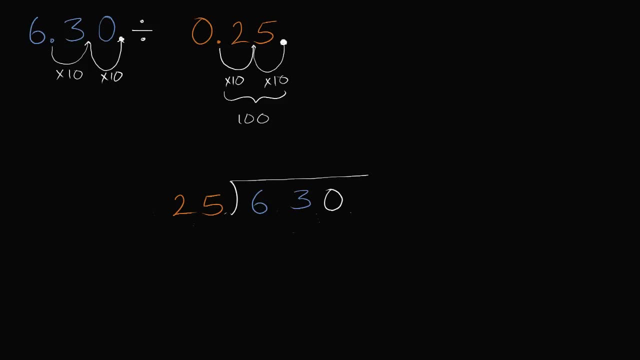 dividing a two-digit number into a three-digit number, And so we could say: well, 25 goes into six zero times. so let's keep going. 25 goes into 63.. Let's see: two times, 25 is 50.. 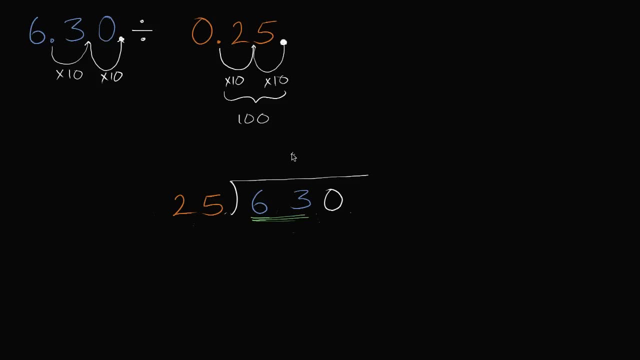 Three times 25 is 75, so that's too much. So we want to go two times. Two times two times 25 is going to be 50. And we can subtract. Or, if you didn't know, two times 25 was going to be 50,. 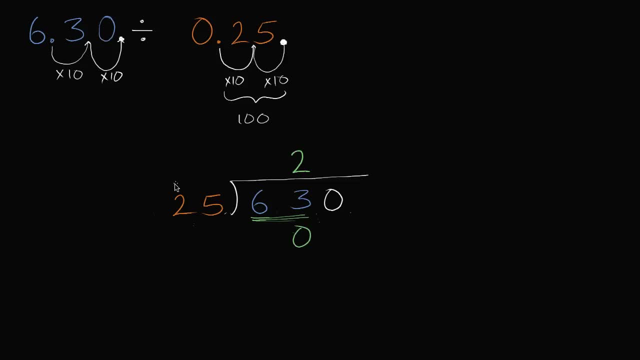 you could have said: two times five is 10.. Carry the one or regroup the one. Two times two is four plus one is five. So we got 50. And now we subtract And we get: three minus zero is three. Six minus five is one. 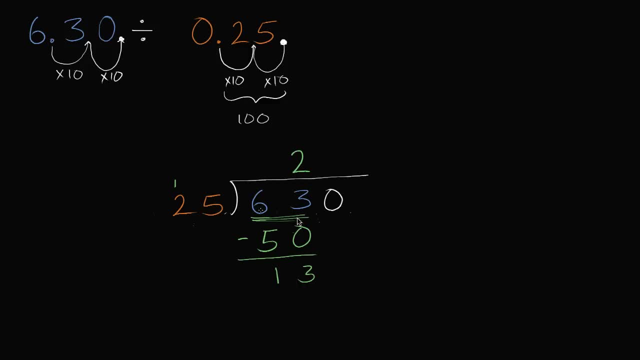 And now we bring down the next digit We can bring down, we can bring down this zero, And we could say 25, and let me scratch this out so I don't confuse myself later: 25 goes into 130. how many times? 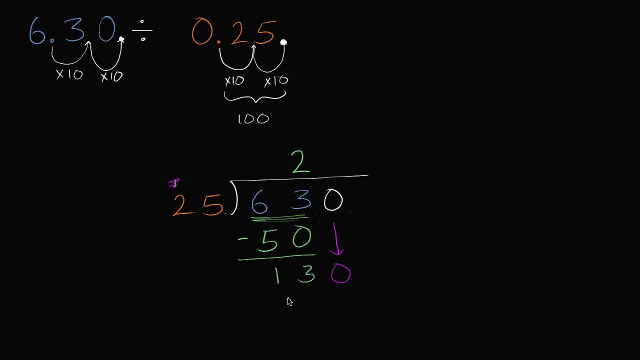 Let's see: 25 times four is 100.. 25 times five is 125.. 25 times six would be 150, so that's too big. So I'm going to go five times, So five times, And I write. 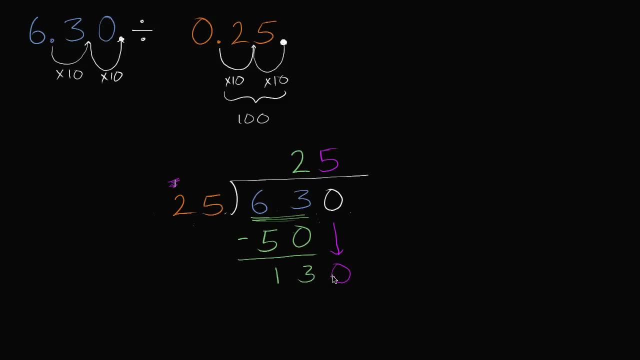 it's very important to keep track of my places right here. I brought down the zero to make the 13 into 130. So when I say 25 goes into 130, five times, I write it above the zero. I write it right above the zero, right over there. 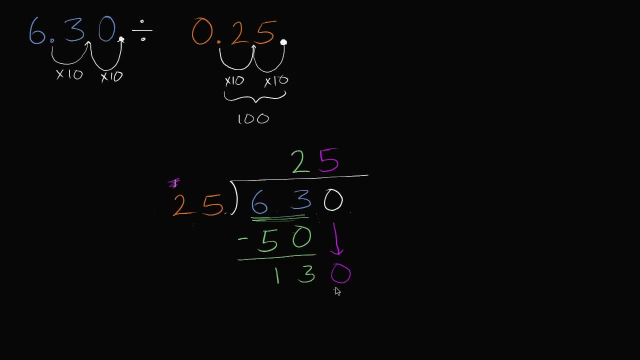 And then five times 25, five times five. we already know what it is, but I'll just figure it out. Five times five is 25.. Regroup the two Five times two is 10 plus two is 12.. And now we can. 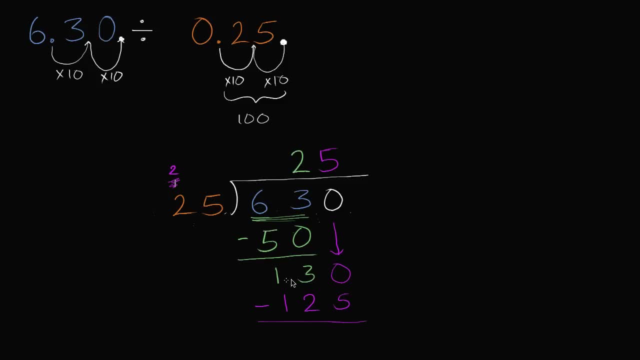 now we can subtract And you might know offhand. well, it is 130 minus 125 is going to be five Or, if you like, you could do a little regrouping, You could make this. you could take a 10 from there. 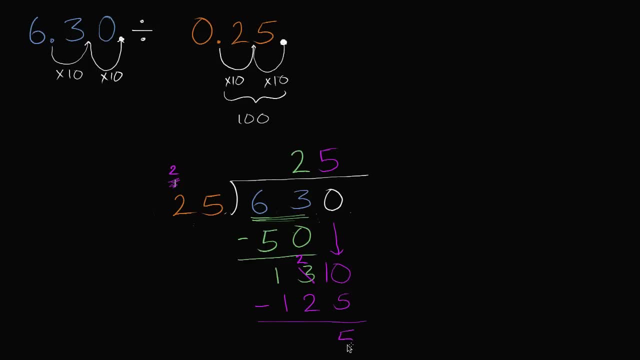 and then put the 10 in the ones place and this becomes 10.. 10 minus five is five. Now we aren't done yet. We want to divide this completely. So we can bring down another zero. We can bring down another zero. 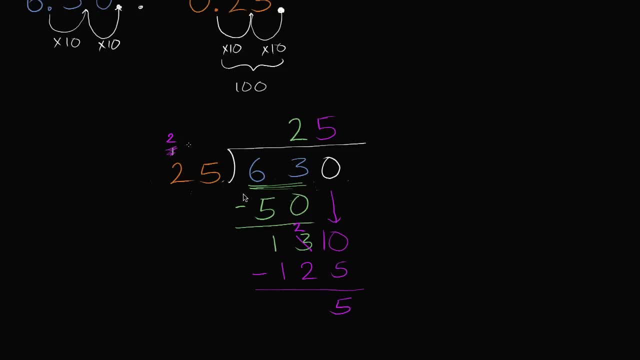 And I'm picking an appropriate color to for the next, so I'll use- well, I already used the green once We'll use yellow, So once again I can bring down another zero, but I have to be very careful here. 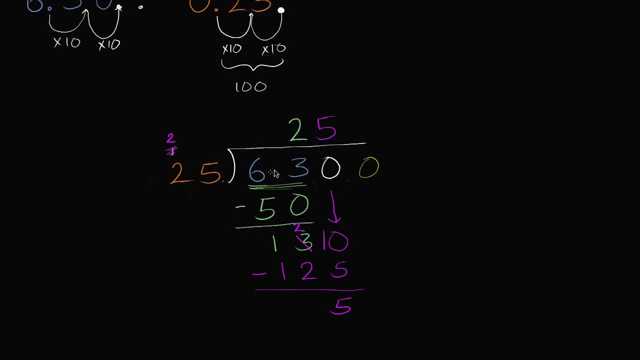 I can't, just, I can't just throw a zero right over there. That's going to turn 630 into 6,300.. I have to be very particular. Say no, look, look, This next zero I'm going to put.